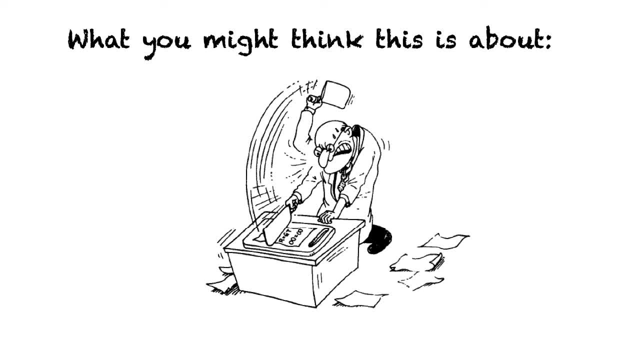 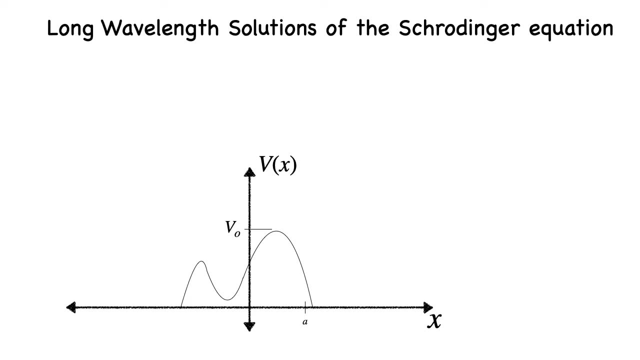 can properly explain. So, in order to find ourselves in this kind of a dicey situation, let's consider quantum mechanics in one dimension with a potential that is short-ranged, Let's call little a the length over which the potential varies, And we will consider probing this potential with quanta of sufficiently long wavelength. 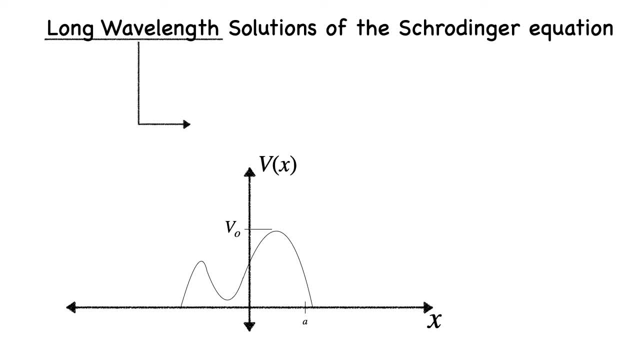 long de Broglie wavelength, which in turn means that we're going to consider quanta with momentum eigenvalues much smaller than A inverse, And the Schrodinger equation here takes the standard time-independent form, with a Hamiltonian given by a sum of kinetics and a 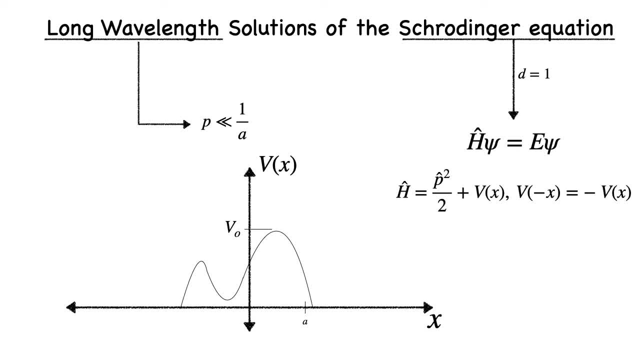 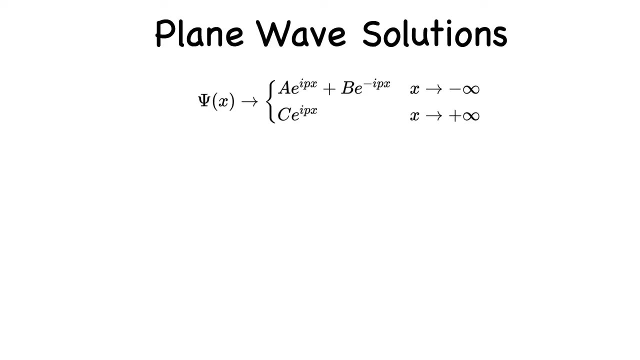 potential and a potential. The particularly interesting case that we'll be considering here will be the one where v is an odd function of space. Normally, where we're given the explicit form of the solution, we will consider an onset of the following form for the wavefunction, And in pictures this looks: 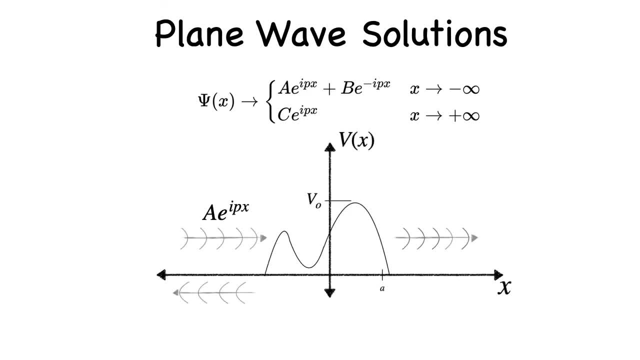 like the following: where we have the following wavefunction: This is the wavefunction that we have in the form of the wavefunction And in pictures. this looks like the following: where we have the some amplitude for an incoming wave, a transmitted wave and a reflected one, 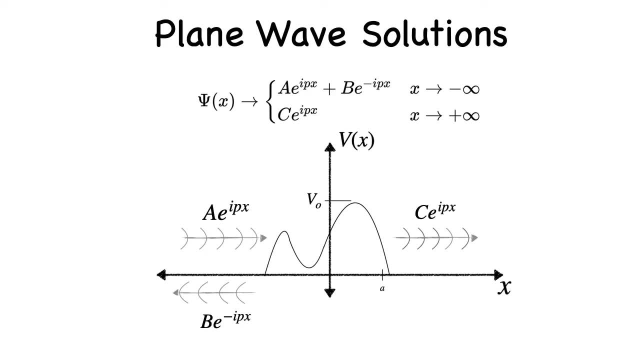 From computing these quantities, these amplitudes- A, B and C- we can infer the transmission coefficient, the reflection coefficient or amplitude, and by unitarity they're related in the following way. So it suffices just to compute one of them. 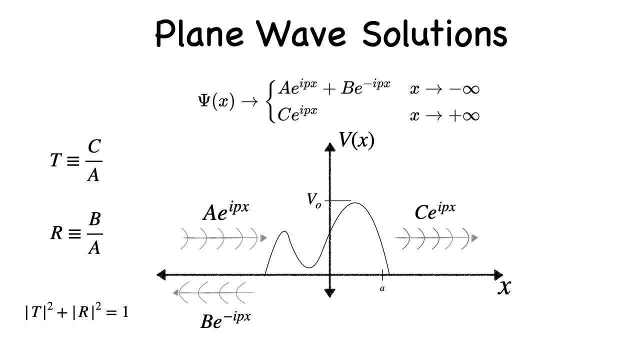 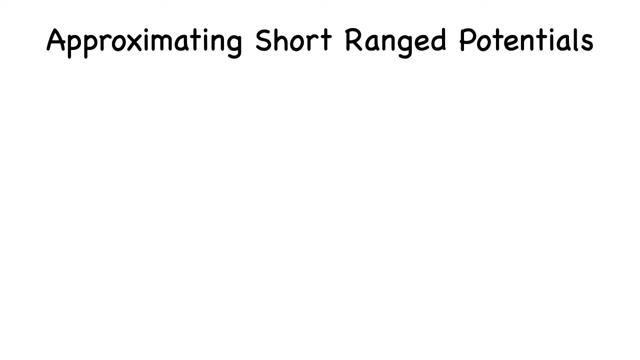 Now by considering waves of de Broglie, wavelength sufficiently large compared to the range over which the potential varies. we might as well approximate these short-range potentials as distributions. Now, where we're considering an even function of space, then we could just use the direct delta function for our distributional potential. 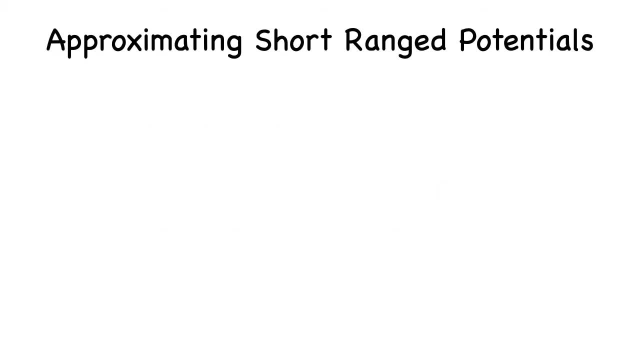 potential. But if we had to consider an odd function of space, then we will need the derivative of the delta function. So a note on what these constants c and c1 are, So we could extract them in principle, where we give it an explicit potential, and did something akin. 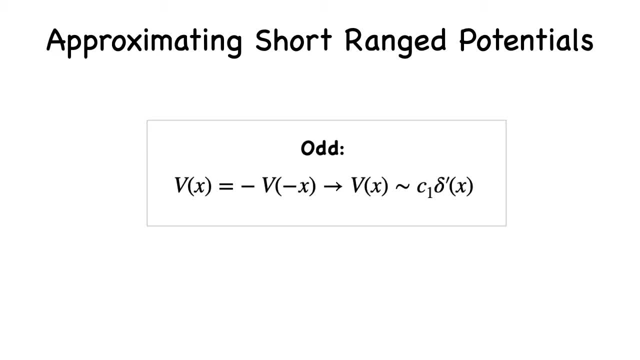 to the multipole expansion in electrodynamics to infer what these are. But if we're to just probe our potential with quanta of very long wavelength, then what we'll have to do is infer them, treat them as coupling constants, like we would in quantum field theory. But 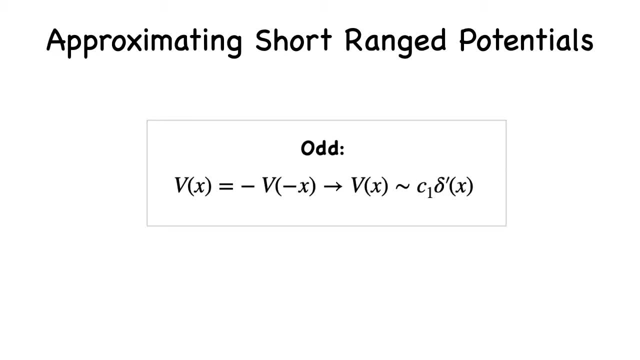 let's plant a flag there and come back to it towards the very end, because the this is an important point. So, to see the issues that arise with an odd function of space being our potential, let's take a look at the S-matrix that describes the kind of scattering that we're interested. 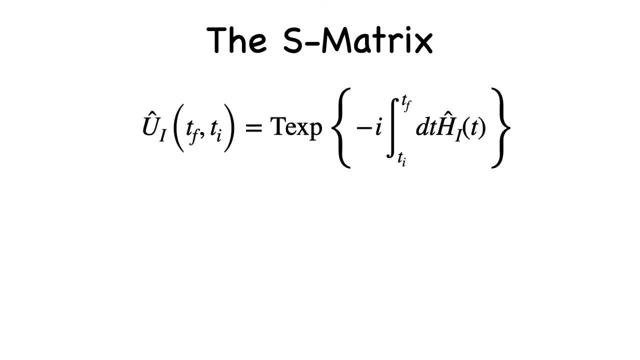 in Now. the S-matrix is related to the following unitary operator that, in the interaction picture, dictates the time evolution of our states. It's given by the time-ordered exponential of the integral of the interaction, Hamiltonian, which is defined in the following way And: 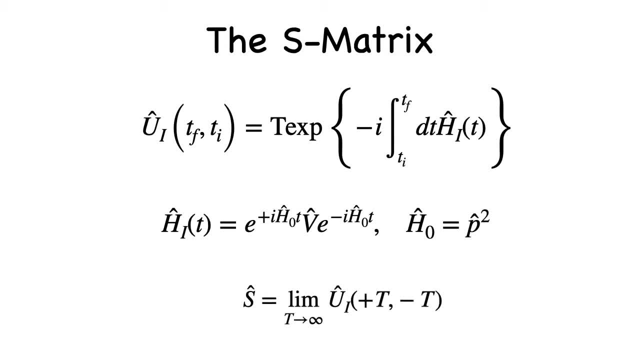 we obtain the S-matrix by taking the interval of time to infinity. So the S-matrix defines the propagation of asymptotic states defined at very early times to those defined at very late times. Okay, And Dyson taught us that we can obtain this quantity in perturbation theory through the: 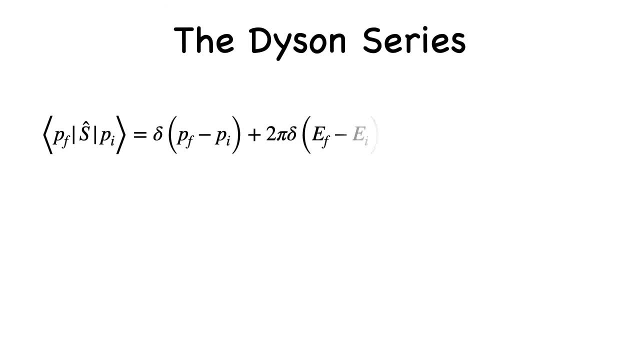 following series. So the leading order contribution is just the matrix elements of the potential, provided energy is conserved. Note that if the potential were zero, if our particles were free, then the initial and final asymptotic states are identical. That just means that. 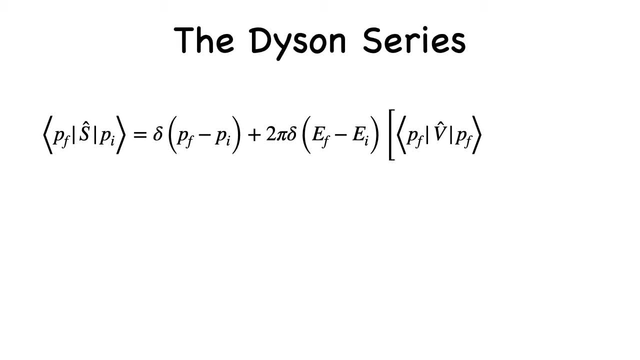 these particles fly right through each other And we have a first or second order contribution coming from the following momentum integral. I'll just demarcate each of these so that we can refer to them in the following slide. So now let's consider what happens when we 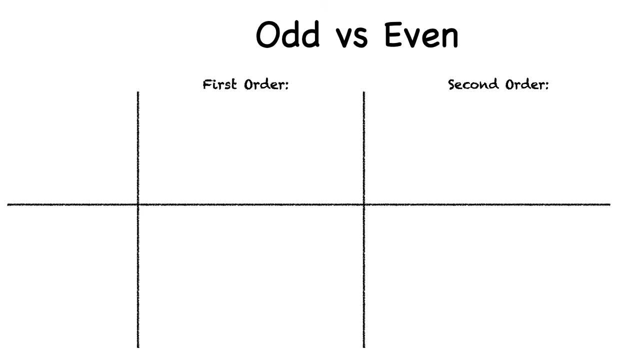 have an approximation for an even short-range potential. The first order contribution gives us a constant. The second order contribution is an integral over momentum that converges. However, if we have an odd potential, the first order contribution is momentum dependent. The second order contribution diverges. 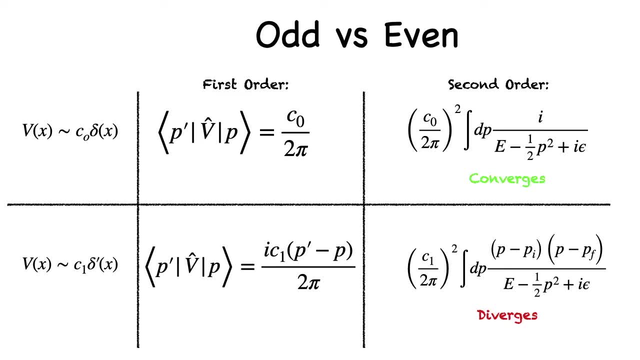 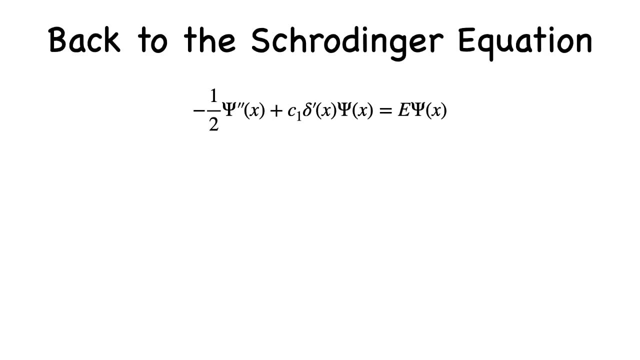 So if we pay close attention to the form of this integral, we'll see that the issue really arises at very large momenta. This breakdown of our Dyson series is reflected in the fact that we could perhaps try and solve the Schrödinger equation with a derivative of delta function potential only to find 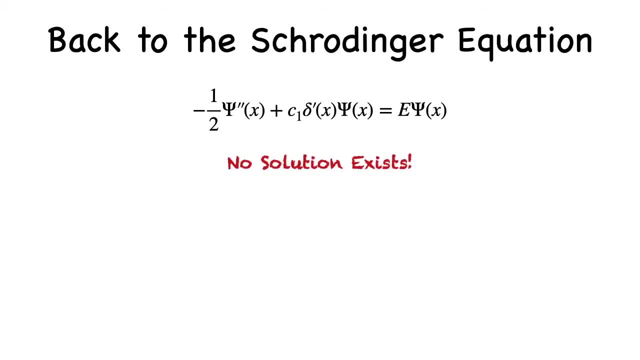 that no solution exists. To see how this is, We can integrate the equation over space around. x equals zero, obtain the following difference equation, and we would normally impose continuity and jump conditions to then go and infer our amplitudes. The issue is that psi prime at zero is ill-defined because it's discontinuous there. 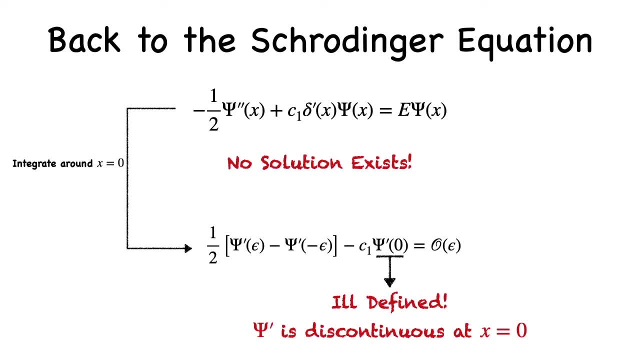 Now we have encountered our simple version of an ultraviolet divergence. So in our example, this issue is an ultraviolet issue because it happens at small length scales, at short length scales or at very large momenta. This is exactly how it would occur in quantum field theories too. 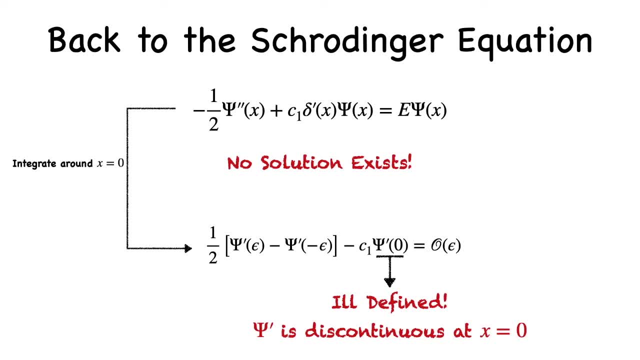 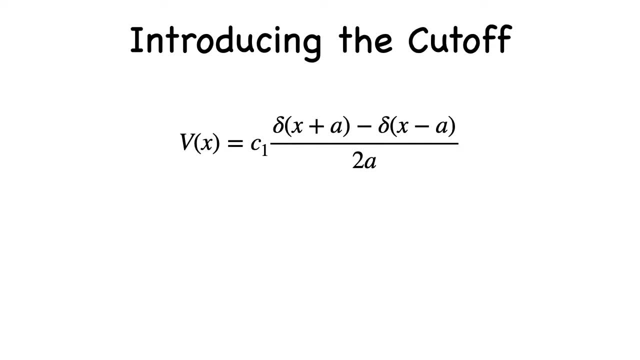 And, like in quantum field theory, what we can do is introduce a short distance cutoff And we can approximate our potential now as a difference of delta functions by introducing this parameter, a. Now, when we take a to zero, we recover our derivative of delta function. 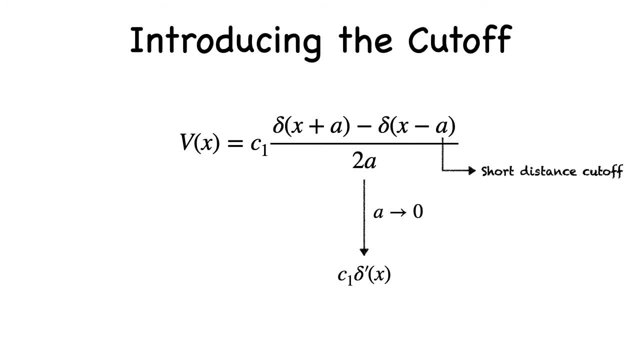 a. here is a short distance cutoff, which I've only named suggestively to be the same as the range over which the potential varies, But it doesn't necessarily have to be this length scale, So long as the wavelengths of the quanta we're interested in are sufficiently large in comparison. 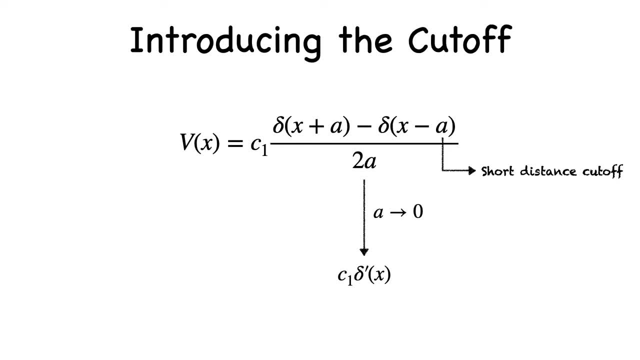 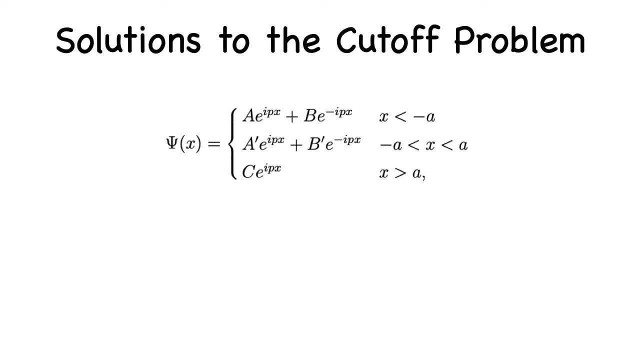 then a could be anything else. So now we can try to make an ansatz to solve the cutoff problem where again we consider some superposition of incoming and reflected waves All the way to the left and in the middle, where the potential varies, we have a different. 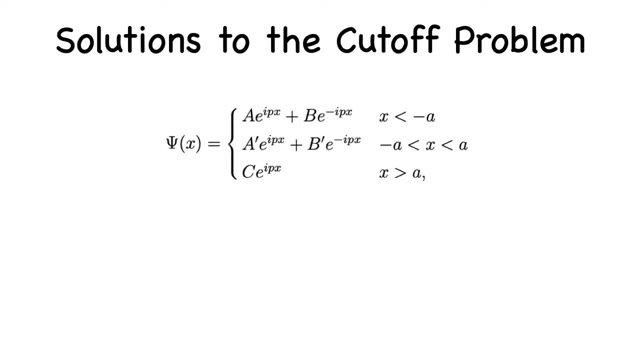 superposition of incoming and reflected waves and all the way to the right we have a purely transmitted wave. Now the curious among the listeners might want to go and do this exercise explicitly and find that 1 over the transmission amplitude is given by the following function of a and: 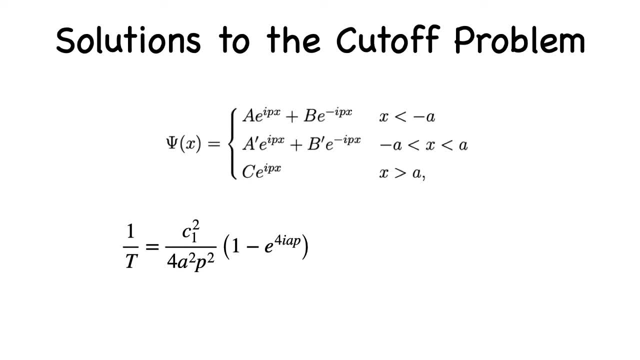 p. Note that this would diverge as a goes to zero, But we could consider momenta that are sufficiently small in comparison to 1 over a and we would find that the transmission coefficient is given by the following ratio: And now we're ready to do the next step, which is the step of renormalization. 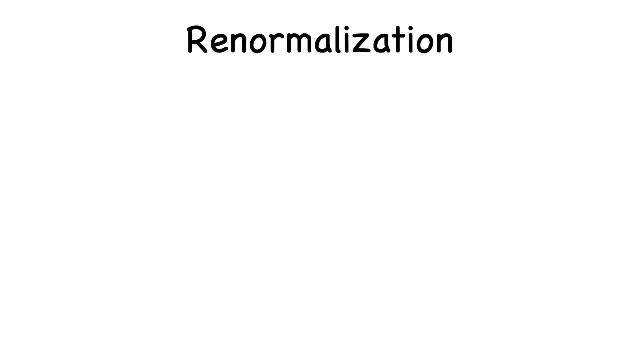 So here we have a drum roll, And we get p, And we get p, And we get p, And we get to just define the ratio of a over c1 squared as c sub r, which is the renormalized coupling, And then we obtain the following result, which is independent of the cutoff: 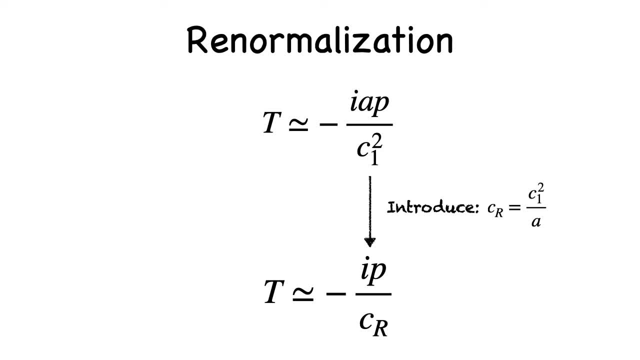 Now we could say that this is a bit bizarre, because all we've really done is introduced another variable. We get p, But the point of C sub r is that we can hold it fixed, provided that we adjust A and C1 in compensatory ways. C1 is something that we would obtain from what we would normally call the. 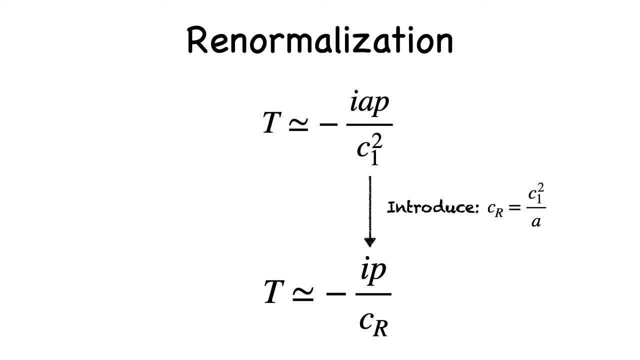 Bayer theory. So we would have to do the expansion, the multiple expansion, of our potential explicitly to find what it is. But if we only had access to quanta of sufficiently low momentum, then all we can really do is infer from the transmission coefficient what C sub r is. 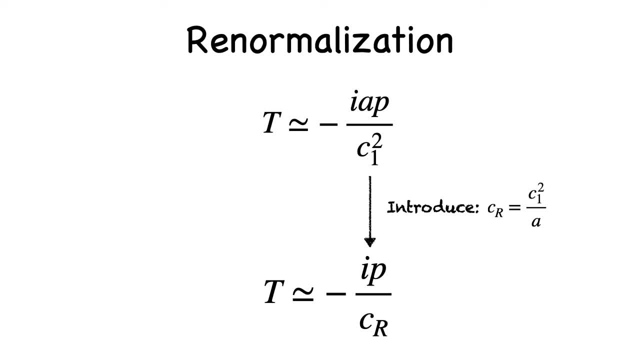 as a phenomenological parameter And then for our purposes, we would be perfectly capable of describing scattering over this potential. So C sub r is really parameterizing the sensitivity of the system to the physics at short distances And furthermore it's an admission of ignorance of the detailed physics at short distances. 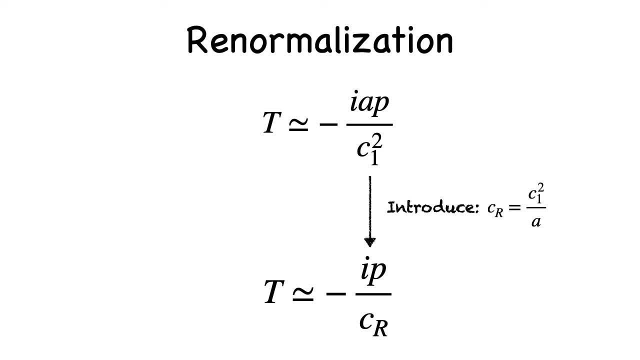 provided we only have quanta of very large wavelength to probe the system with, in particular very large in comparison to this cutoff. So really, renormalization is not so much about cancelling infinities as much as it is about a sort of relativity of scales. 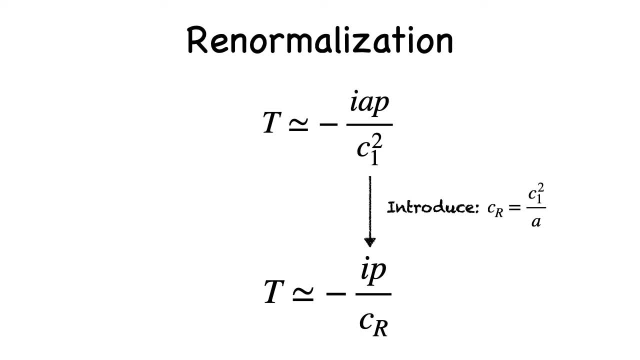 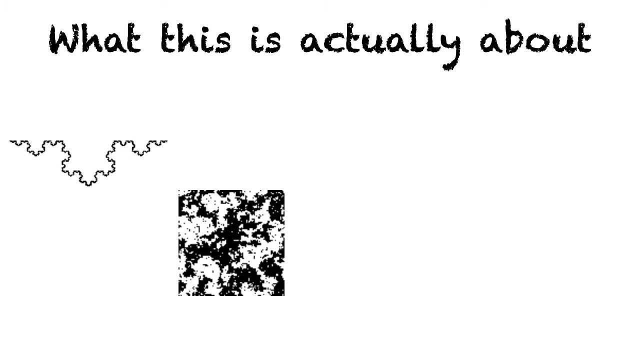 And that perspective was really brought to us from the study of critical phenomena, where all of a sudden, we find that systems no longer care about the scale at which you probe them, start to see scale invariant behavior And, in particular, the kinds of models you would encounter in your education are those like 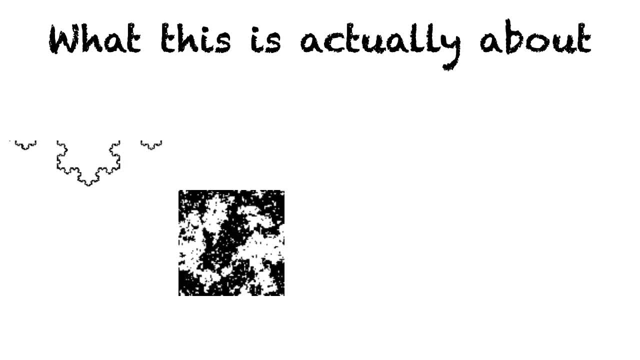 the Ising model and you can try and look at phase transitions that they exhibit and near the critical point. in particular, second-order critical points- is where you start to see this behavior of scale invariance emerging And, of course, there is a high-energy physics. 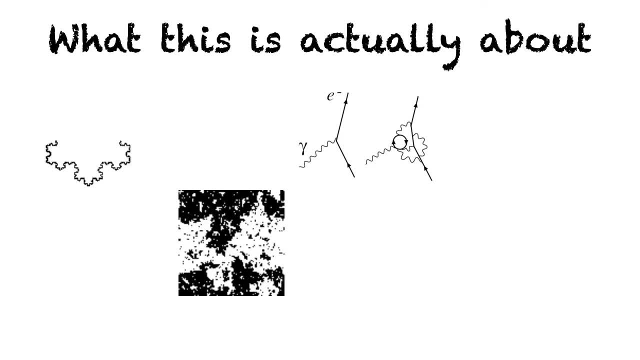 um parallel to all of this, which is that our running coupling constants describe how interactions are screened as we vary the energy of the particles that are undergoing scattering. And really how we can make sense of this procedure of renormalization comes from thinking. 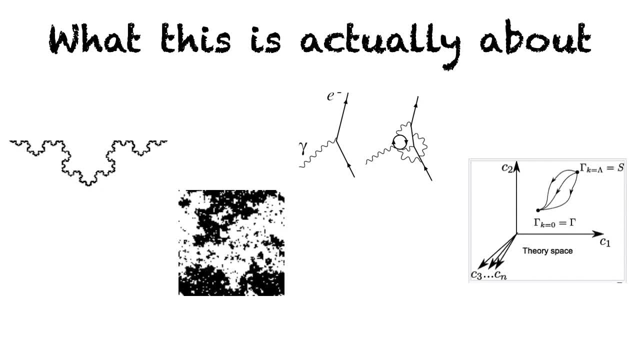 about certain renormalization group flows. As a result, we can say that linear randomization is a very useful theory, which is a very useful method to understand the space of theories, which applies very broadly across statistical mechanics, quantum field theory and high-energy physics, and even astrophysics and cosmology.